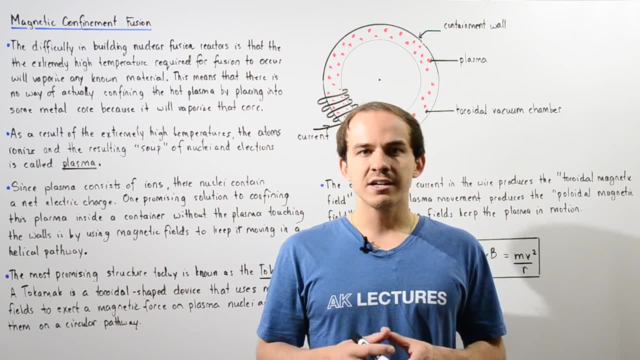 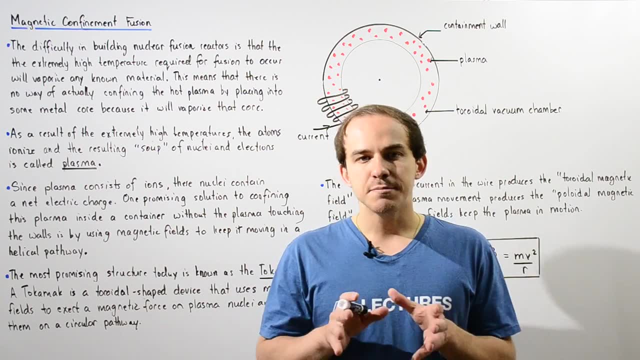 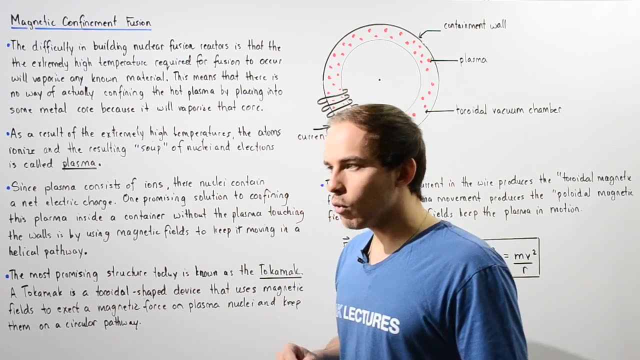 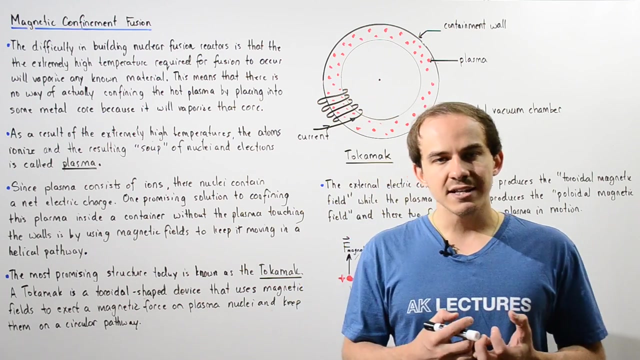 In our discussion on nuclear fusion reactors, we said that no known fusion reactors actually exist on earth today, And that's because of the difficulty that is involved in creating or building and sustaining our nuclear fusion reactor. So, basically, in order for fusion to actually take place, we have to have a very high density of reactants, a very high density of fuel. 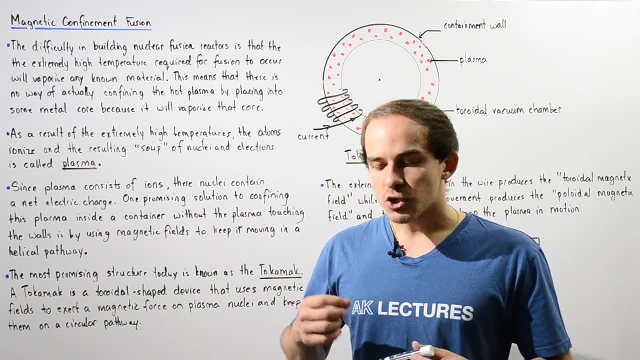 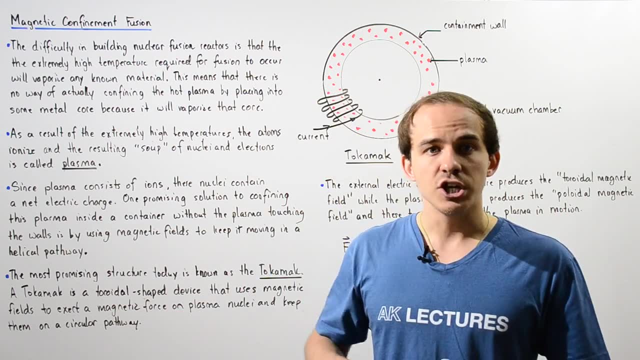 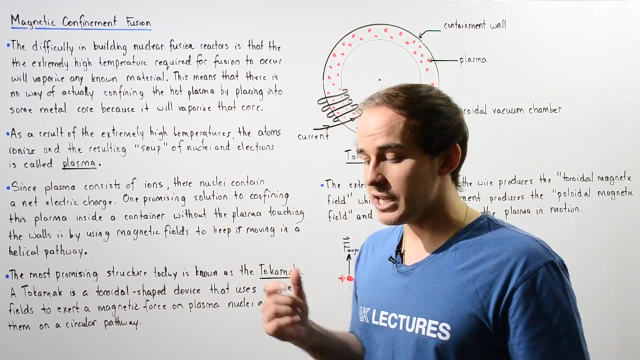 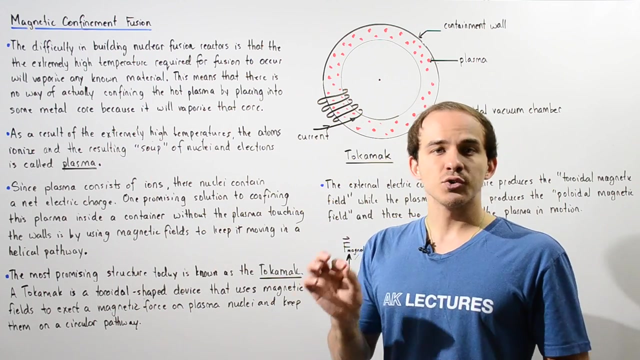 and very high temperatures. So basically the high temperatures give those nuclei a high enough kinetic energy for them to combine or fuse, to form our more stable nuclei and release our energy in fusion. The problem is when we increase the temperature to that high amount. as a result of that high temperature, any known metal, any known material? 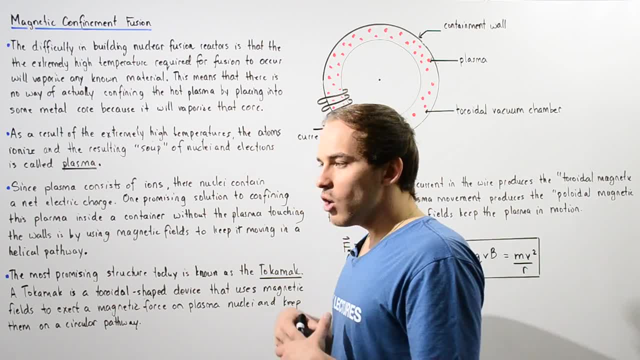 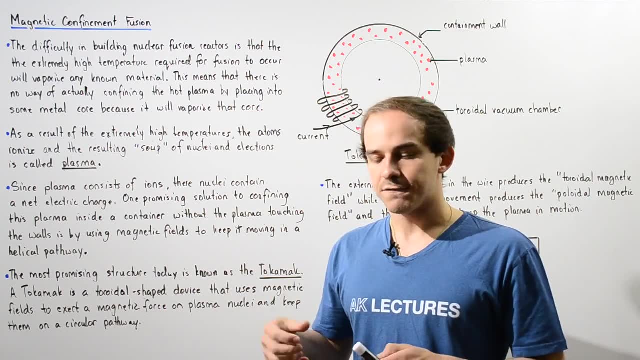 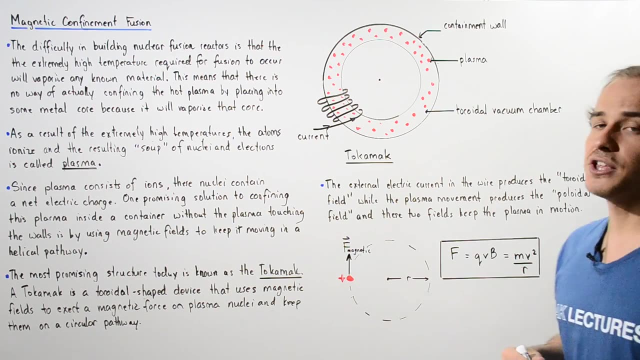 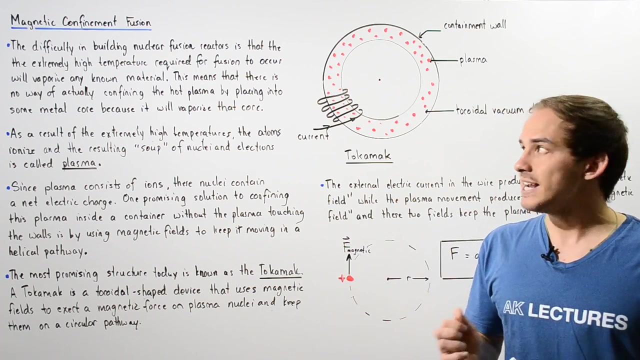 will readily vaporize, And so we have no way of actually containing that plasma that is required for fusion to take place. So the difficulty in building nuclear fusion reactors is that the extremely high temperatures required for fusion to occur will vaporize any known material. This means that there is no way of actually confining the 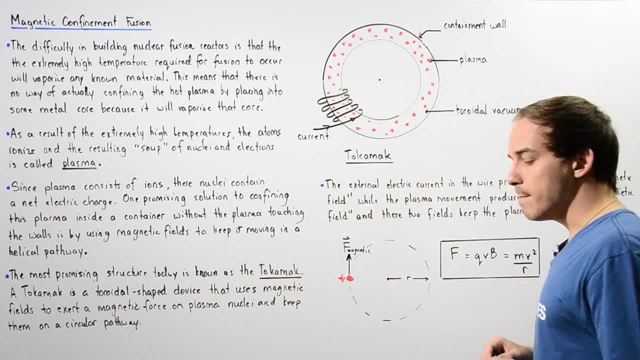 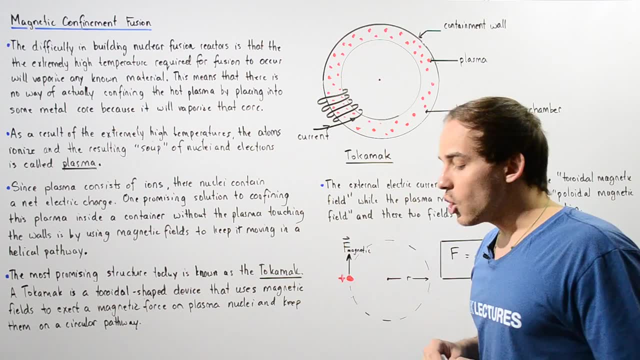 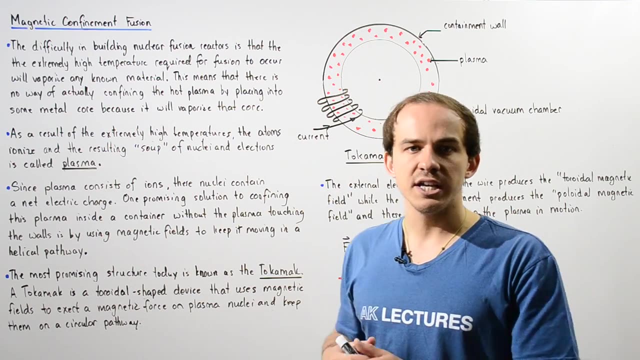 hot plasma by placing it into some metal, because that plasma will vaporize that metal core. So what exactly is plasma? So whenever we take a bunch of nuclei and we heat the nuclei to a certain temperature, to a certain high temperature, we heat the nuclei to a certain temperature. 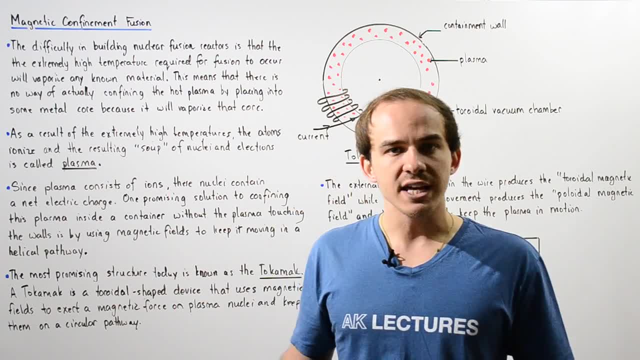 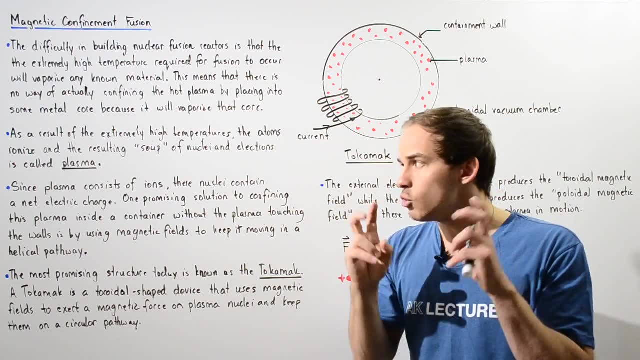 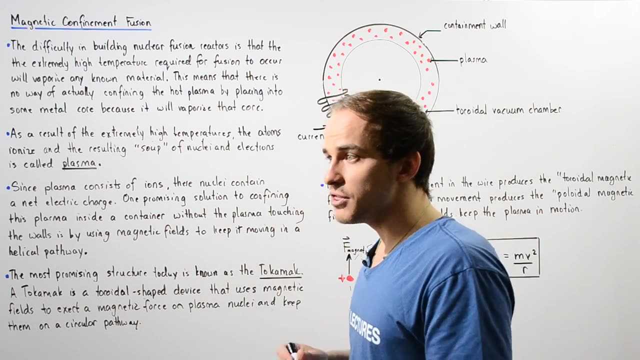 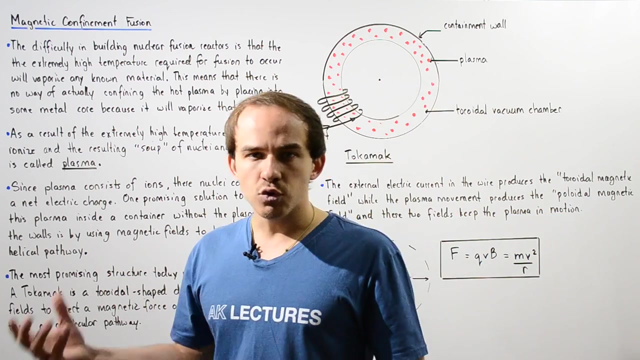 we basically ionize those nuclei and create a soup of nuclei, ions and electrons, And this entire soup is known as plasma. For example, the sun consists mainly of plasma. That's because the sun is at a very high temperature. That high temperature readily ionizes the nuclei on the sun. 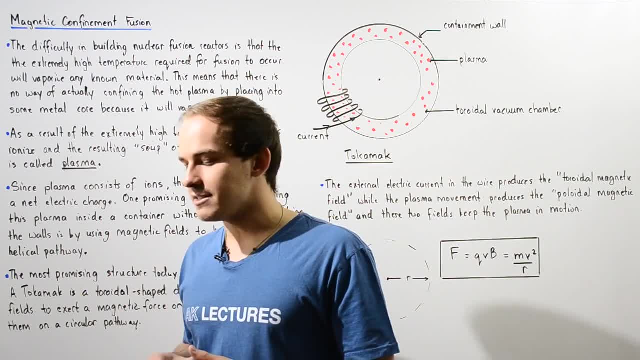 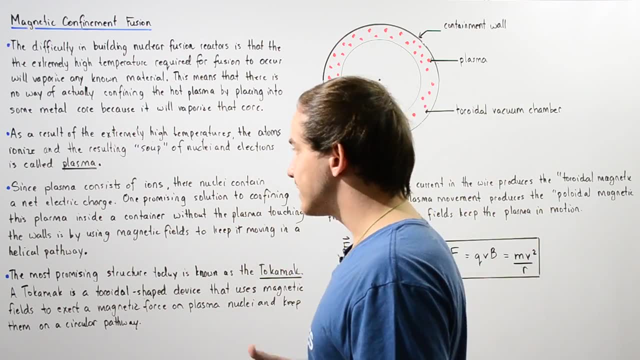 And that allows fusion to readily take place. So it's possible. That's when the Favorites bulb of the sun is at medium temperature, And the way we reach the subgrade is that the plasma sits on the sun. So in a way we can think of the sun as being a nuclear fusion reactor. 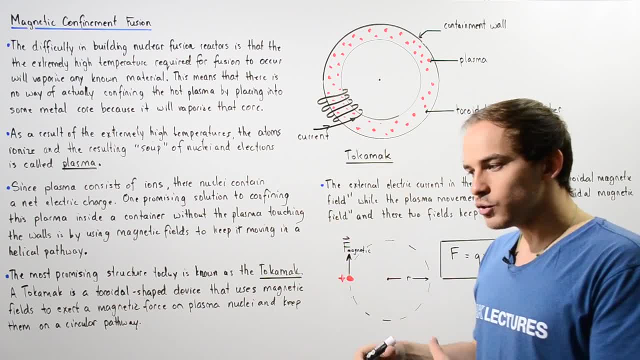 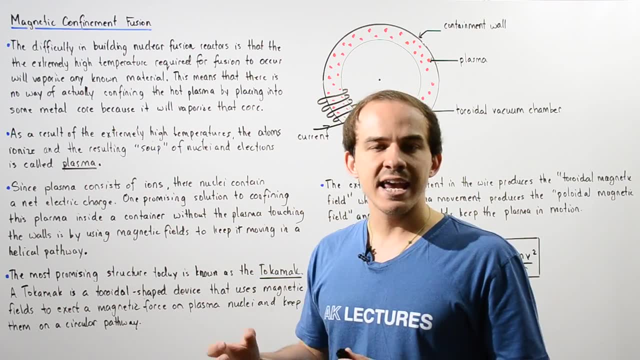 Now how exactly can we actually create a, Finally chamber that actually contains the plasma? So, take it away, there's a So, since plasma consists of ions. these nuclei contains electric charge, And so that means one promising method of containing our plasma in the gas. If you've ever tighten your astronauts dificulties, we have a connection to the nerves inside your joints. It's very cool because we know thesetawa pieces don't set offeng a plasma level And so that tree lying in the final 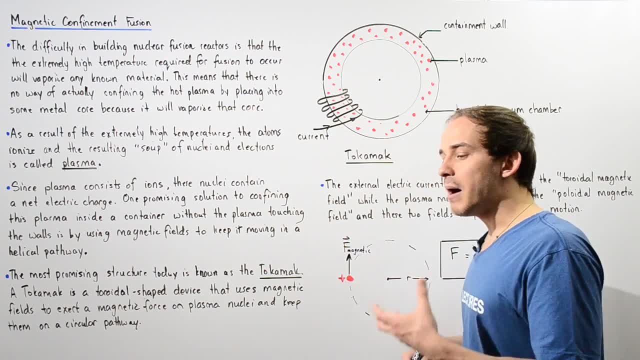 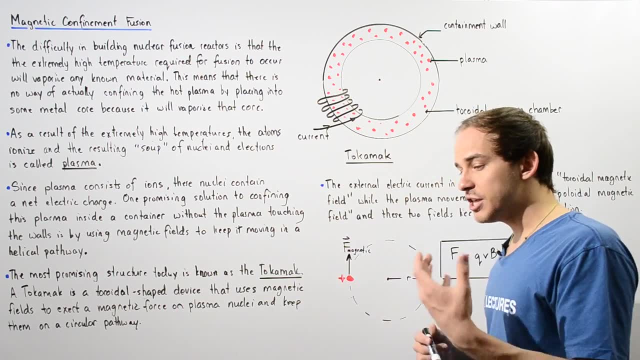 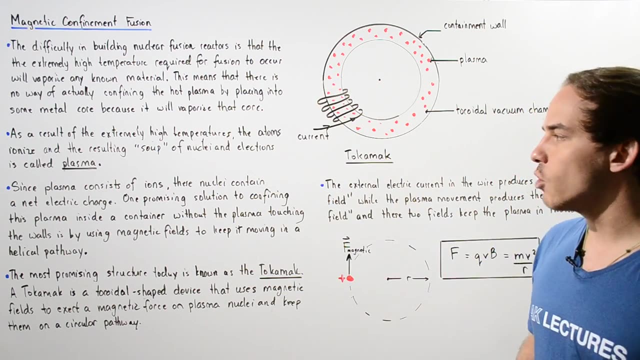 inside some type of container is by using magnetic fields to actually guide that plasma around that container, within that container, without actually touching the walls of our container and vaporizing it. So, once again, one promising solution to confining this plasma inside a container without the 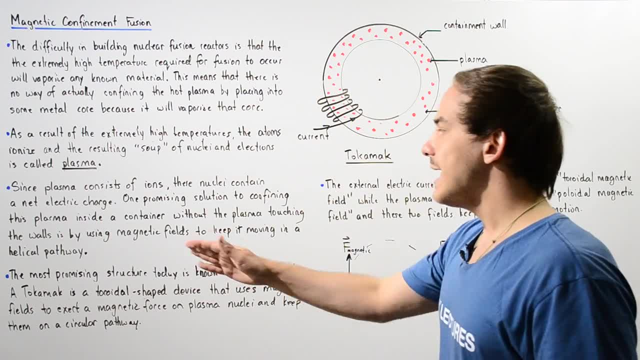 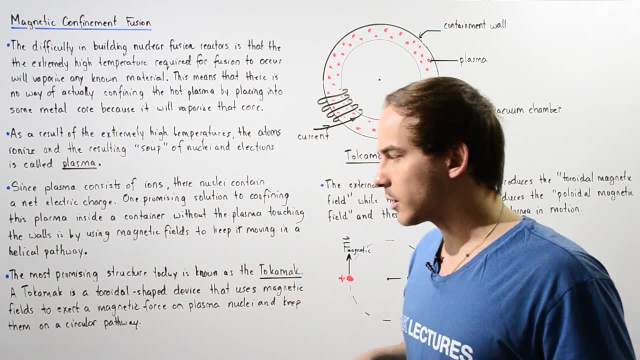 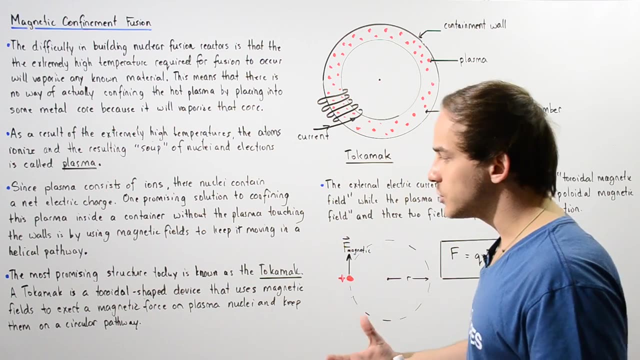 plasma touching the walls and vaporizing. it is by using magnetic fields to guide and keep the plasma moving in a helical or circular pathway. Now the most promising structure that was initially developed by the Russians and later perfected at Princeton is known as the tokamak. 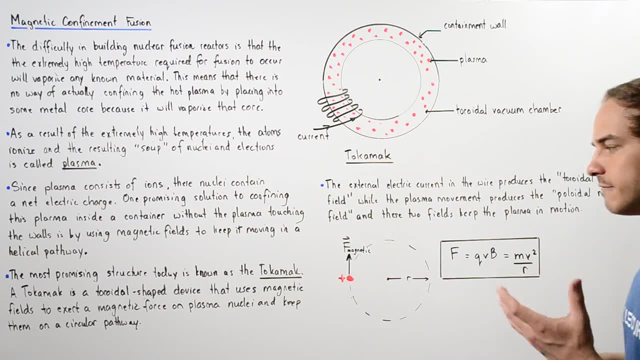 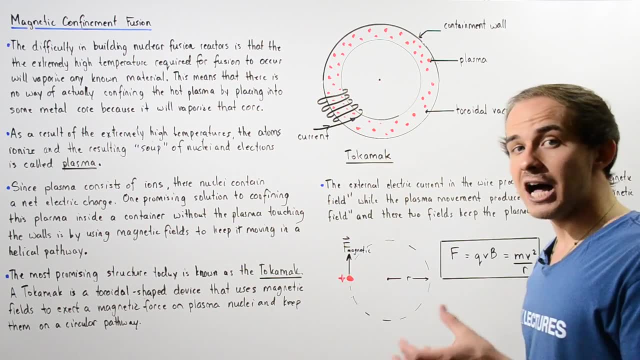 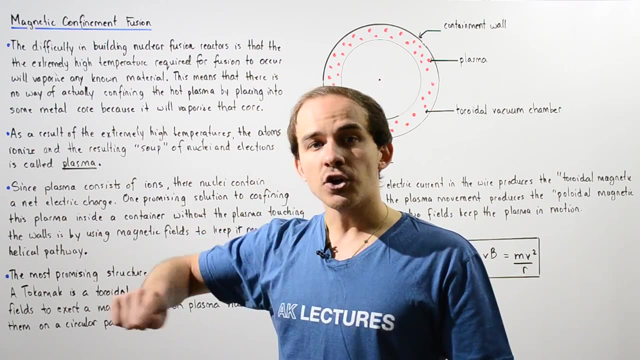 A tokamak is basically a toroidal shaped device that uses two types of magnetic fields. A tokamak is a magnetic field to exert a magnetic force on the plasma ions, on the plasma nuclei, and keep those ions circling that container in a helical pathway. 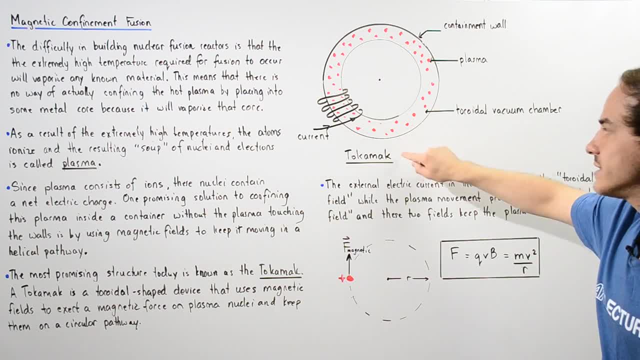 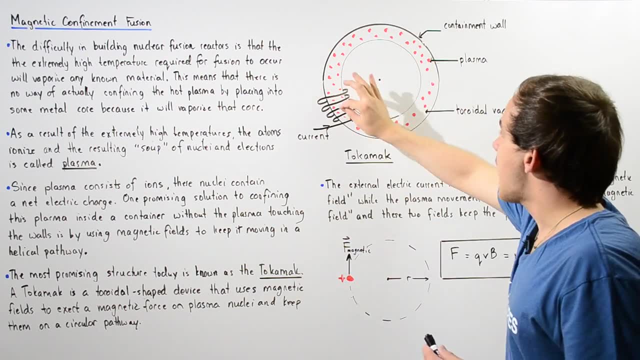 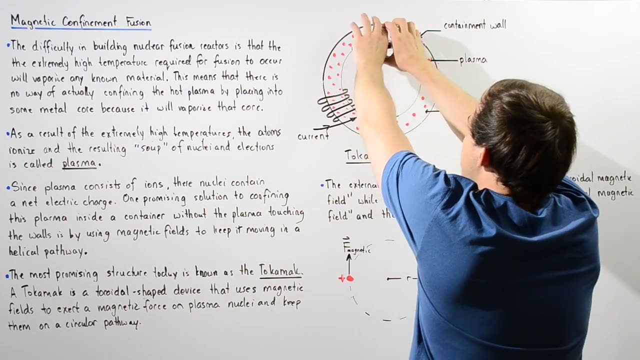 And this is shown in the following diagram. So this is one example of a tokamak. So we basically have our ions and electrons, our plasma, inside the following containment walls. So this is our containment wall and this inner region is known as the toroidal vacuum chamber. 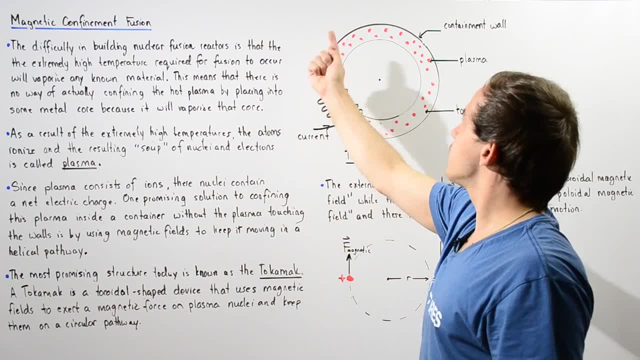 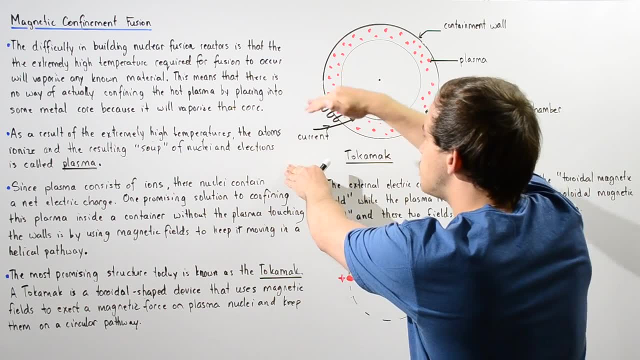 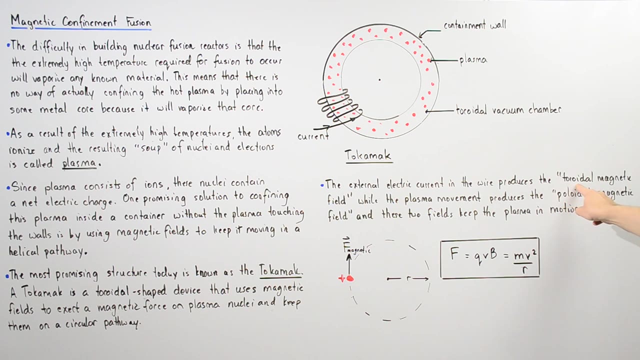 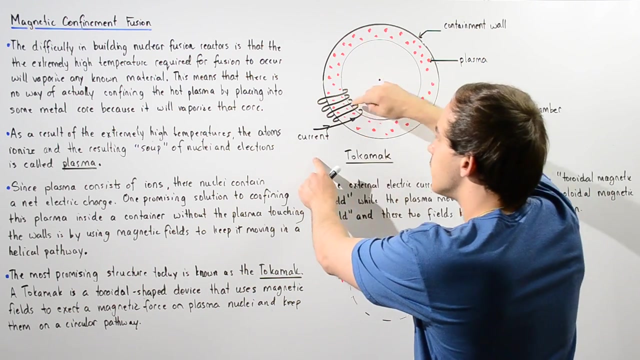 So we basically have a conducting wire that loops all the way around the entire chamber and the external current that moves inside this chamber basically exerts a certain magnetic field. This magnetic field is commonly known as the toroidal magnetic field. Now, the movement, The movement of the plasma around as a result of this magnetic field created by the current. 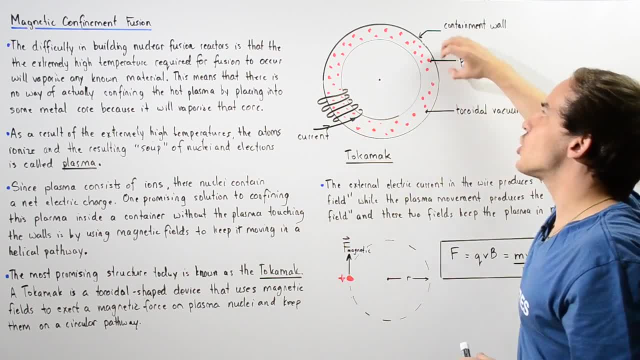 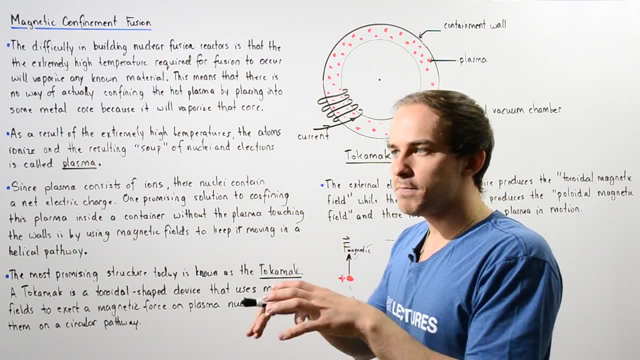 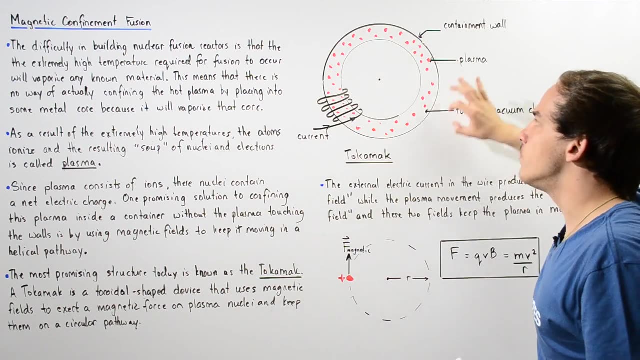 moving in this wire basically creates its own magnetic field that we call the poloidal magnetic field, And these two magnetic fields basically interact to create the magnetic force that acts on the plasma particles to keep them moving in a circle. So recall that any time we have a magnetic field, 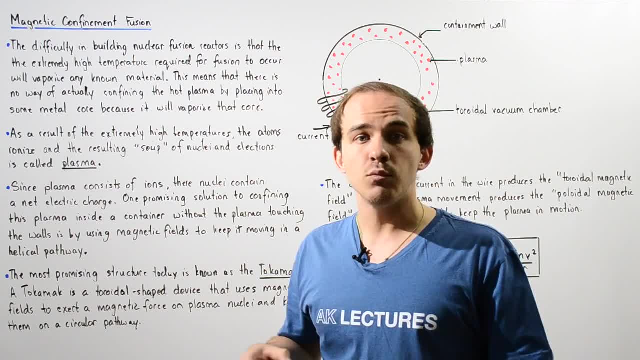 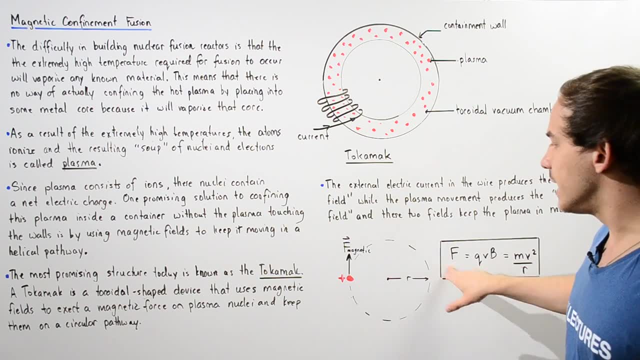 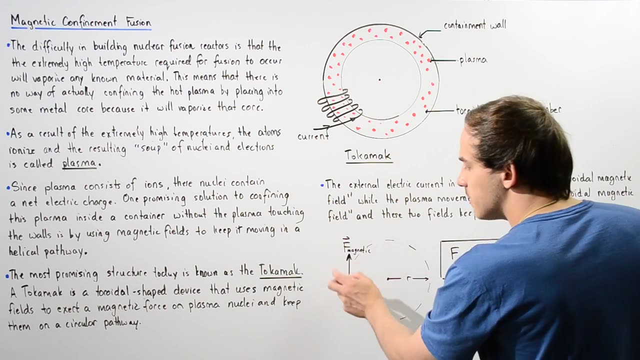 So we call it the toroidal magnetic field. Any time we have a magnetic field B and we have a charge Q that is moving in some fashion, the magnetic force that acts on that particle. for example, let's take one plasma ion with a positive charge- the magnetic field acting on this particle as a result, or the magnetic 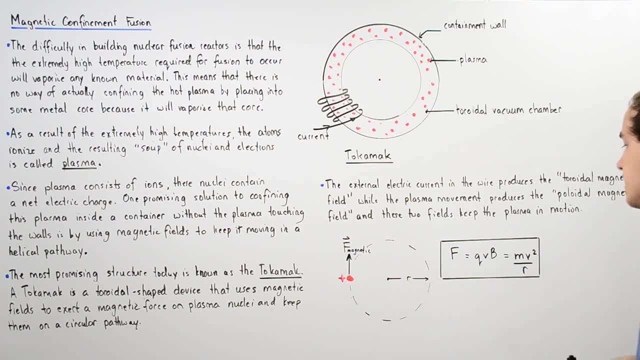 force acting on the particle as a result of the magnetic field B is given by this equation, where Q is the charge and V is its velocity. So the magnetic force acting on this particle is given by this equation, where Q is the charge and V is its velocity. 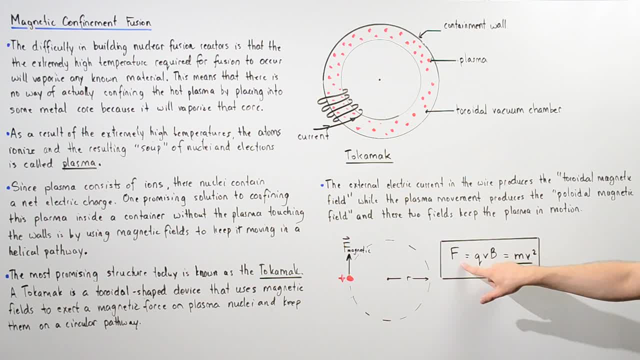 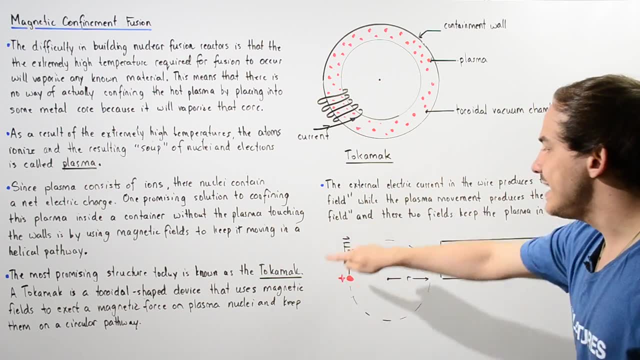 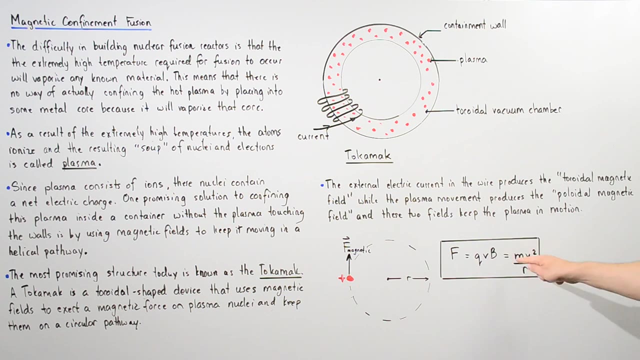 So the magnetic force is equal to Q times V times B, And if we are to keep the plasma rotating in a circular fashion, that means this force- the product of these three quantities must equal to M, V squared divided by R. So basically, V is once again the velocity and 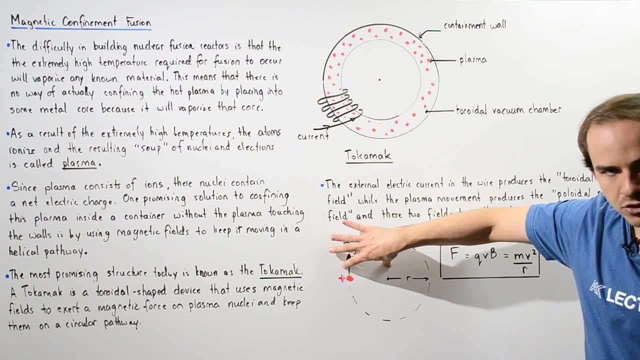 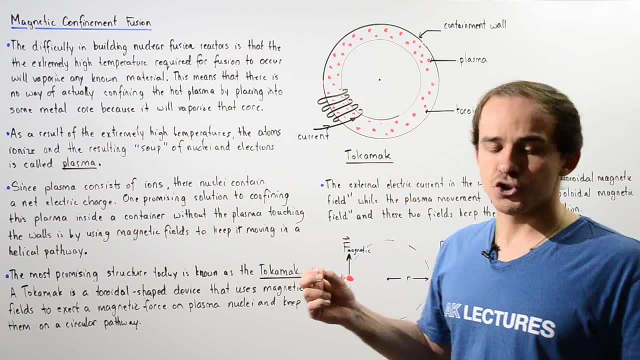 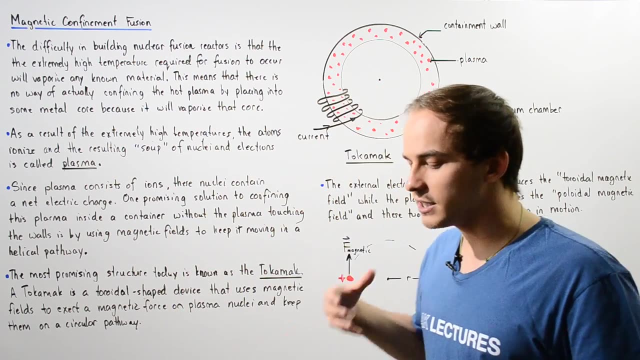 R is the radius of this helical pathway. So once again, it is very simple. It is very simple. It is very difficult to actually create our fusion reactor because if the plasma inside that reactor actually touches the walls of our container, it will readily vaporize it. 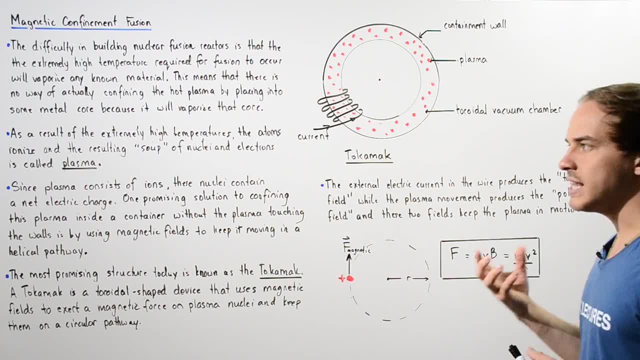 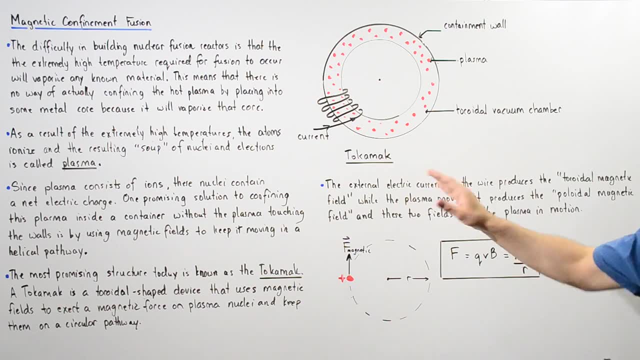 So to keep the plasma from touching the walls of the container, we have to use some type of magnetic field. So we use this device, known as a tokamak, that actually allows the plasma to move around in a circular fashion without touching the walls of our container.